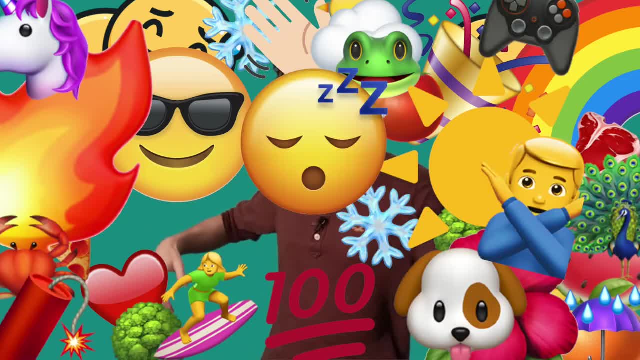 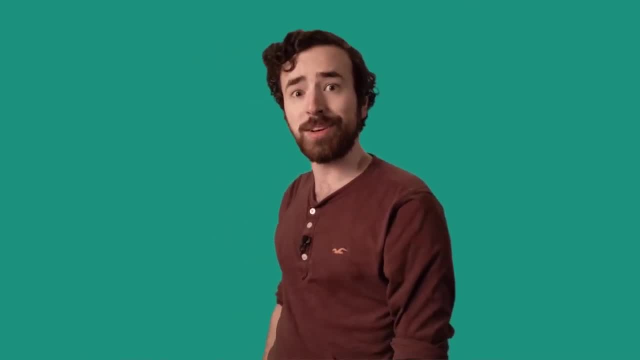 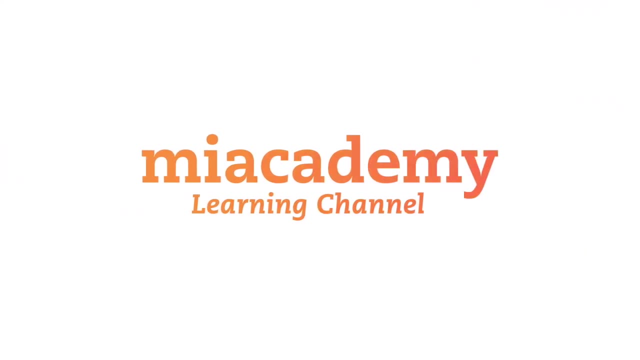 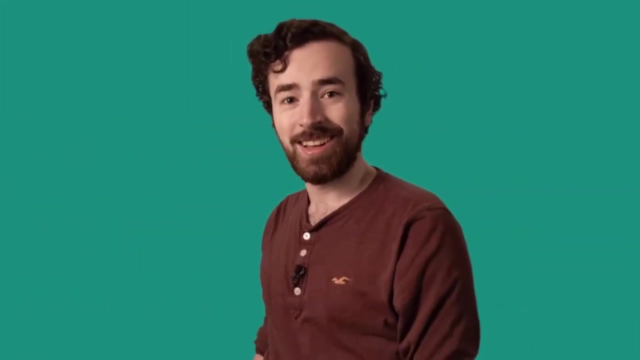 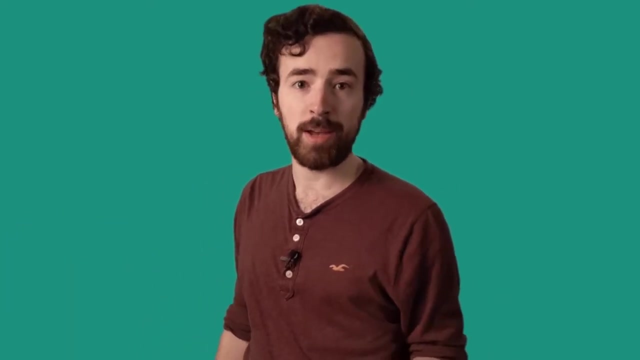 sunshine and fire, and dog and flower and sleeping and clown and professor and fruit. That is an enormous amount of emojis. So I bet you're wondering: what do emojis have to do with maps? Well, today we're going to learn how to read a map, And you can read a map by using the map key, And the map key gives us symbols. 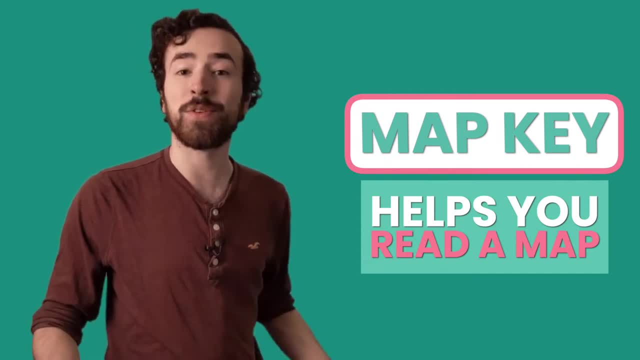 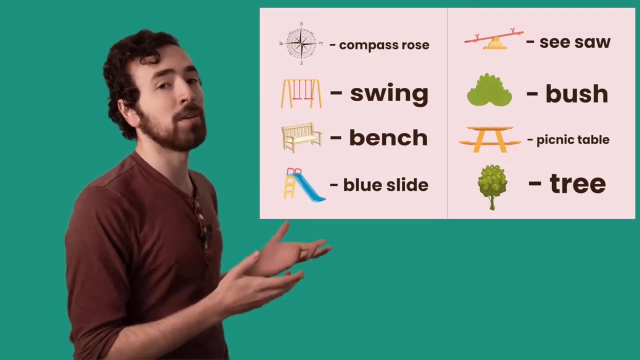 much like emojis that tell us information. It helps you read the map and lets you know what you're looking at. This is an example of a map key. Now you already know a fancy map skill word. that's on this map key. 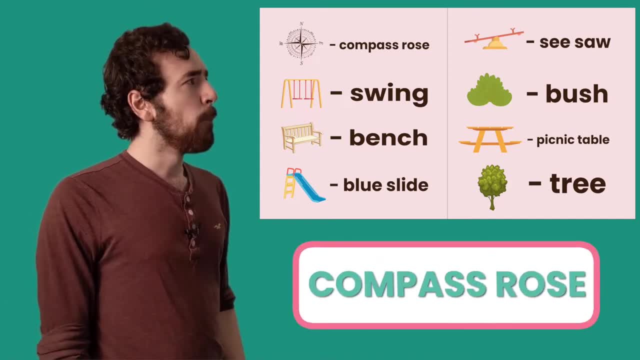 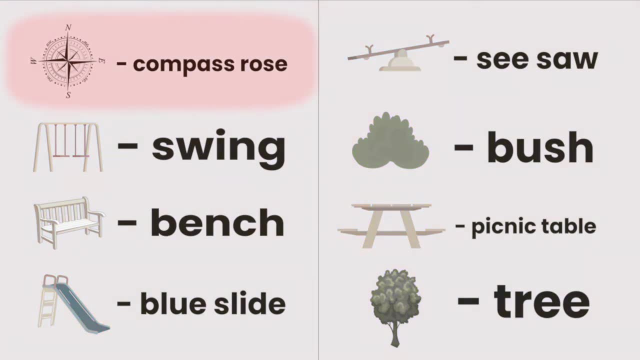 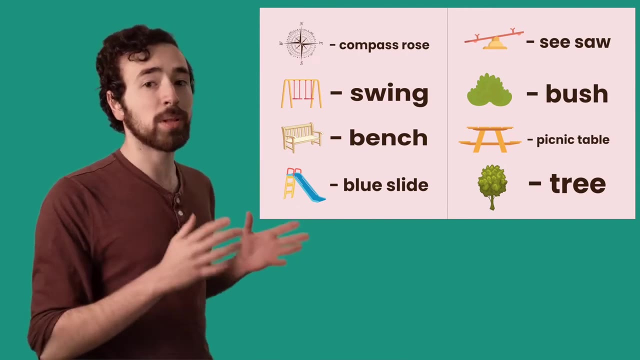 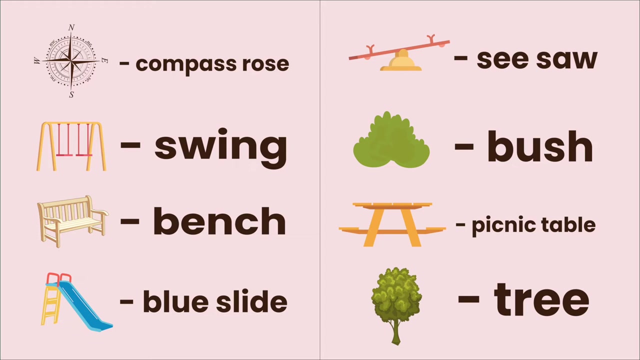 the compass rose. Can you help me find the compass rose on this map key? Oh, there it is, Thanks. Now let's look at some of the other symbols. These are special places and things that are on the map. So let's say, you want to have a picnic at the park. We'll want to go to an area that has picnic. 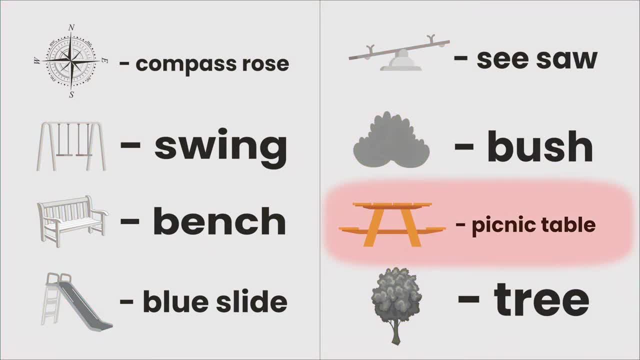 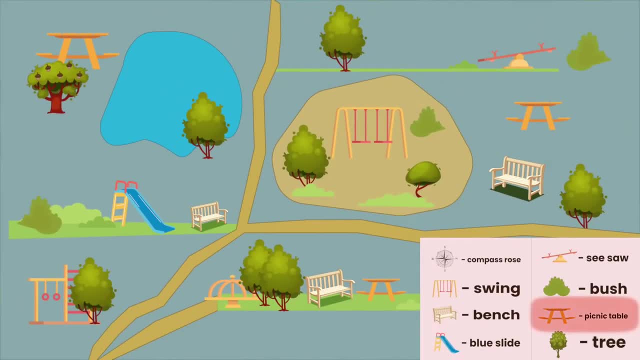 tables. Here's the picnic table symbol in our key. It looks like a picnic table right Now. let's look for the picnic table symbol on our map. Wherever we see this symbol, we'll know that it's an area with picnic tables. It doesn't. 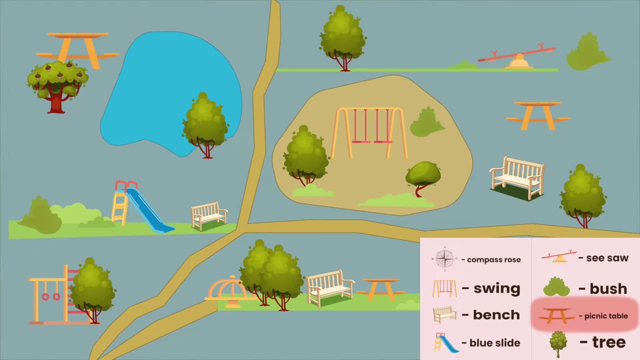 mean there's just one picnic table there. It means that the area is what we're looking for: A picnic table and a picnic table. with picnic tables. It's so much easier to read a map when you use the key to find the things you're looking for. I have an idea. Let's use our map key. 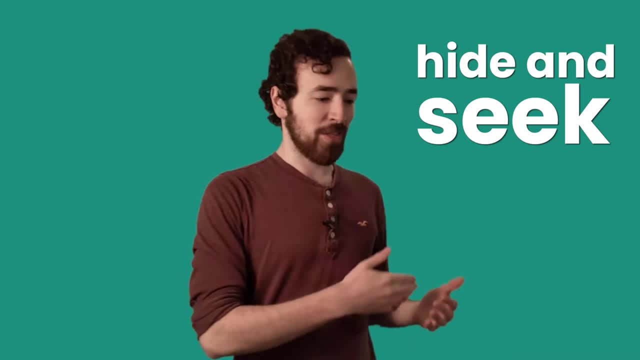 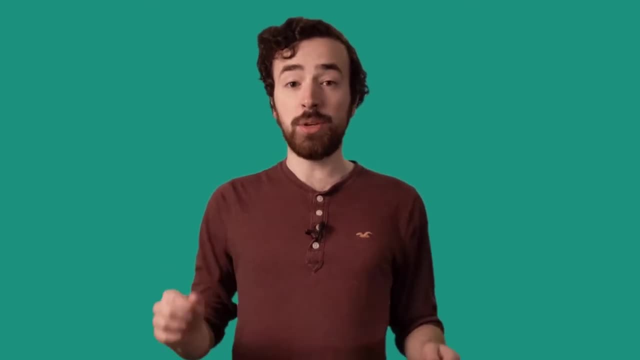 skills to play a game of hide-and-seek. I've got three mischievous puppies that are gonna go hide in the park and leave us clues to know where to find them. Let's use our map key skills to follow the clues and find the puppies. Are you? 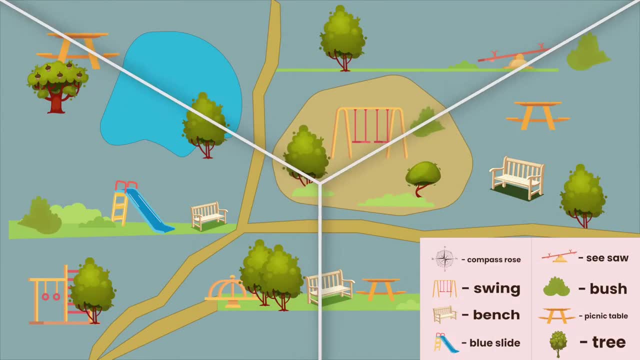 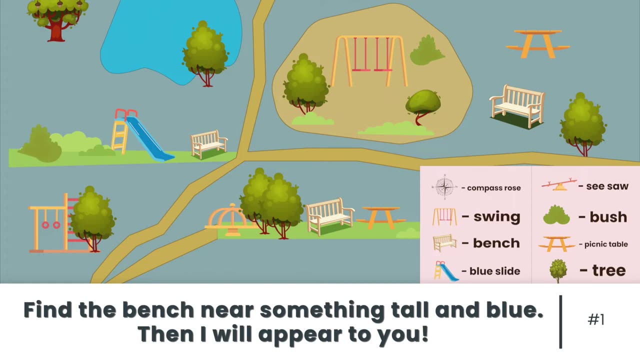 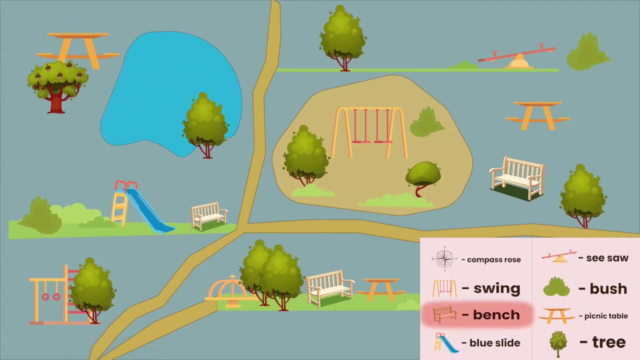 ready, Here we go. Alright, here's our first clue: Find the bench near something tall and blue. then I will appear to you. Okay, let's look for a bench in our map key and something tall and blue. Oh, here's one, A slide. Okay, now let's find. 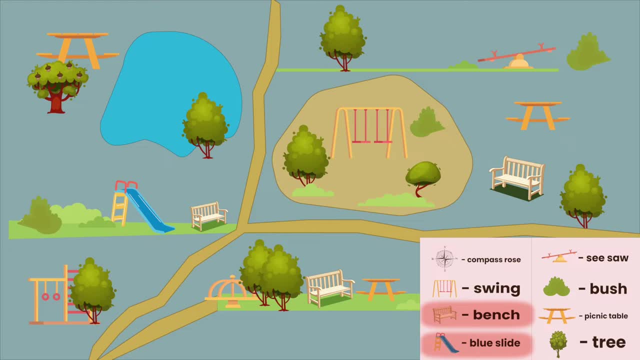 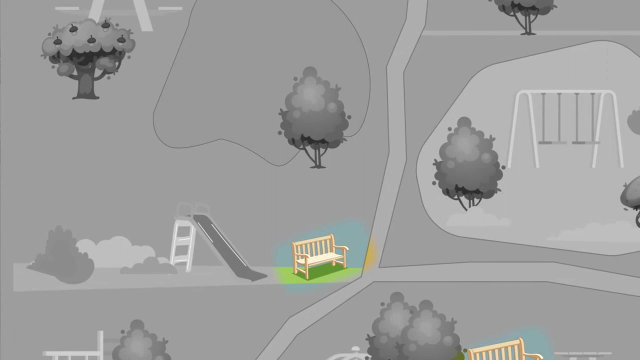 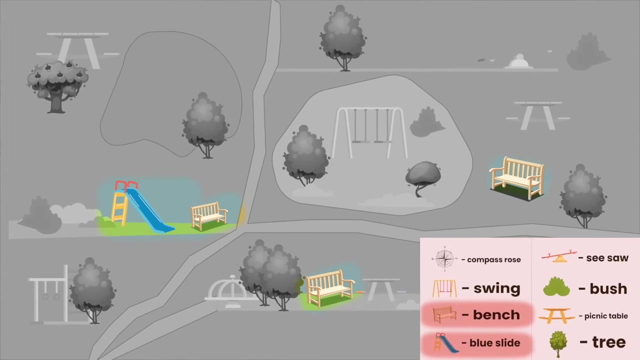 benches on our map. Clap loudly to let me know when we find one that is near something tall and blue. Oh wait, Thank you, I almost missed it. Good job, This bench is next to something tall and blue. It's a slide. Now that means our. 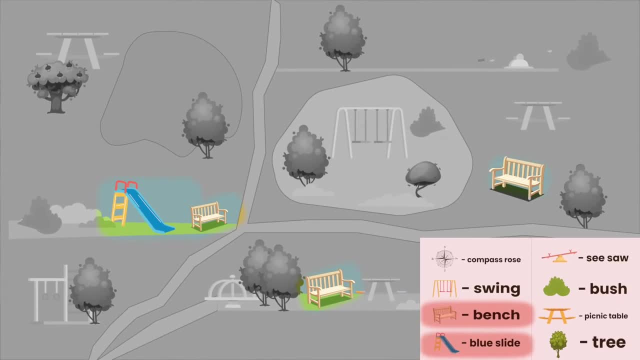 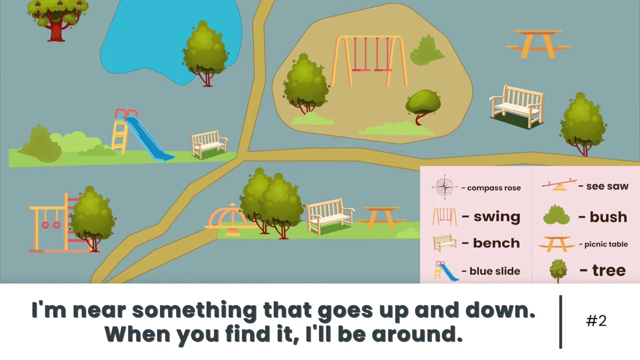 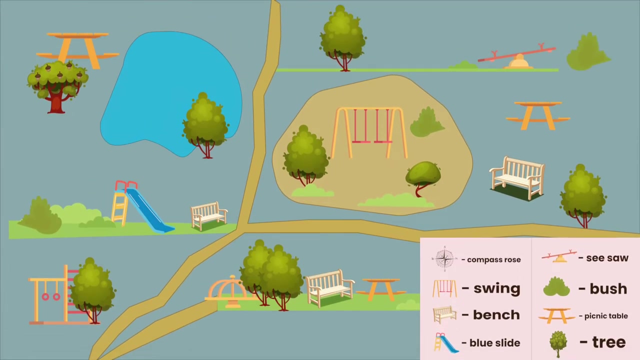 puppy is hiding somewhere around here. There's puppy number one. Great job. Now the second clue. I'm near something that goes up and down. When you find it, I'll be around. Do you see a symbol on our map key that goes up and down? I see two. 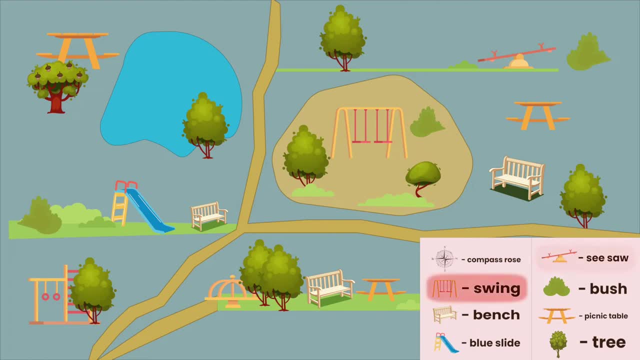 things Swings go up and down and the seesaw goes up and down. Let's look together for the second puppy. Jump up and down when you find him. Here's the swing on the map. See it matches the swing in the key. Hmm, No puppy here. Let's go find the. 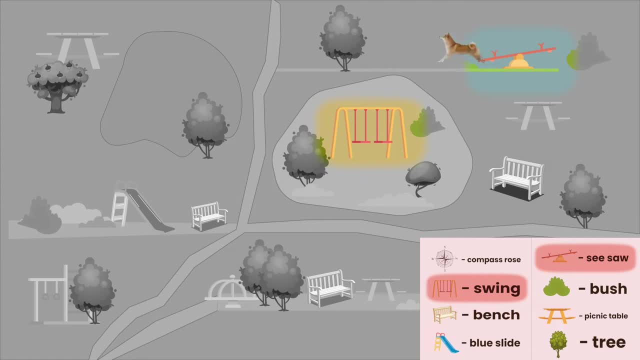 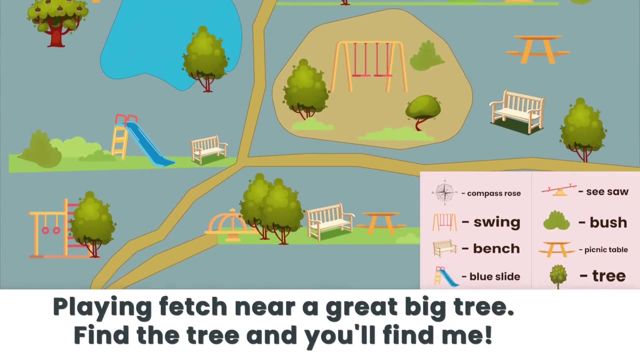 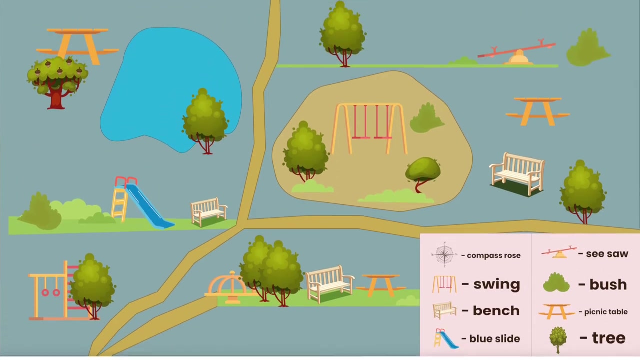 seesaw Puppy. Great job. Now we'll look for the third and final puppy. Here's the clue: Playing fetch near a great big tree. Find the tree and you'll find me. This is the symbol for the tree in the map key. Now let's find the tree on the map key. 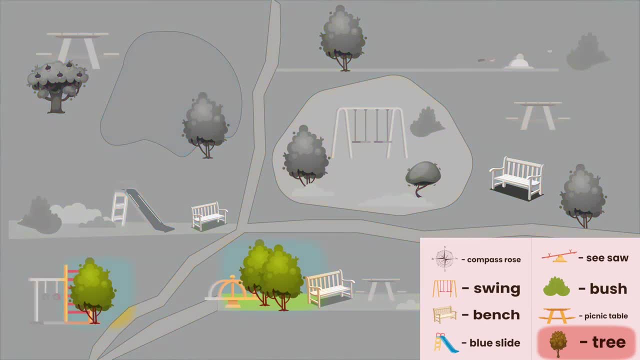 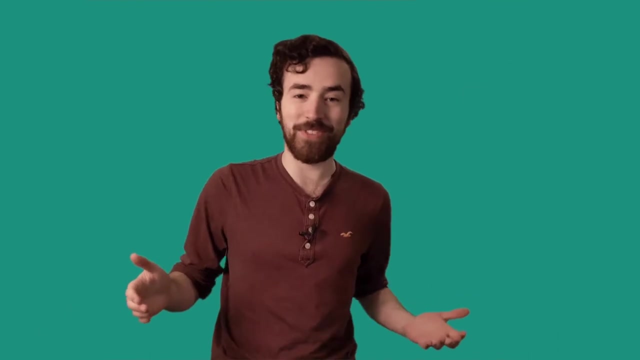 We should find the third puppy. Shout the word puppy when you find him. There he is. We found the third puppy right by the tree, just like the clue said, You did a great job finding all the puppies and it's because you read the map key and looked for the symbols.